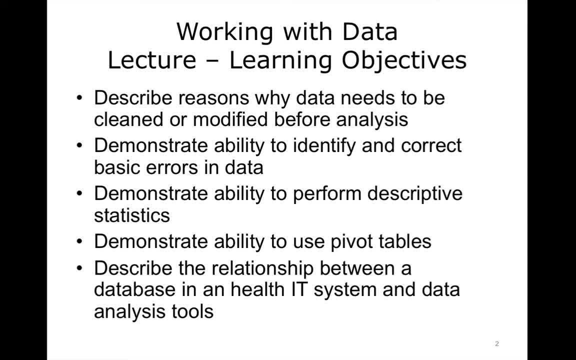 describe reasons why data need to be cleaned or modified before analysis. demonstrate the ability to identify and correct basic errors in data. demonstrate the ability to perform descriptive analyses. demonstrate the ability to use pivot tables and describe the relationship between a database and a health IT system and data analysis tools. 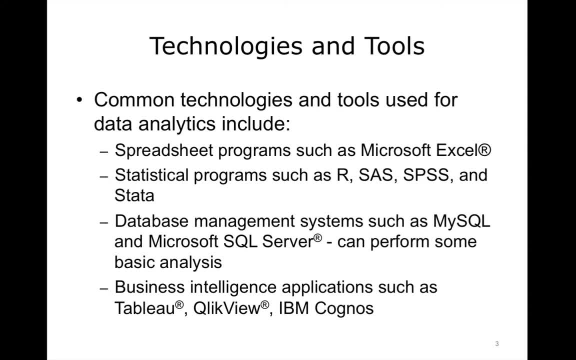 Common technologies and tools used for data analytics include spreadsheet programs such as Microsoft Excel and dedicated statistical programs such as R, SAS, SPSS and Stata. Note that database management systems such as MySQL and Microsoft SQL Server can be used for data analysis. 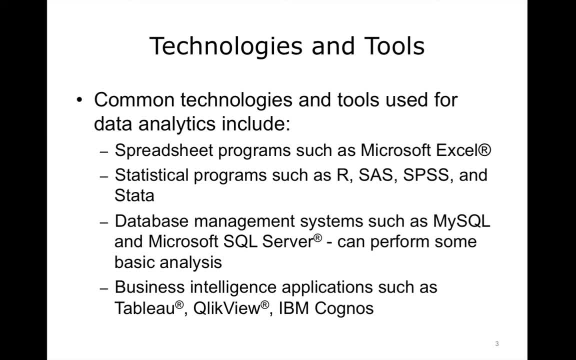 They can perform some basic analysis, but this is not their strength. Typically, data will be retrieved from a database, such as an EHR's database, using a SQL query. The data will then be imported into another application for the statistical analysis. 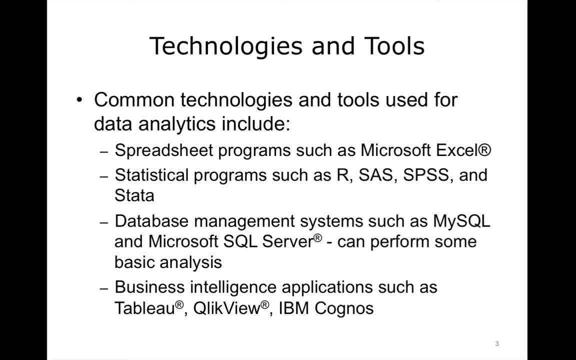 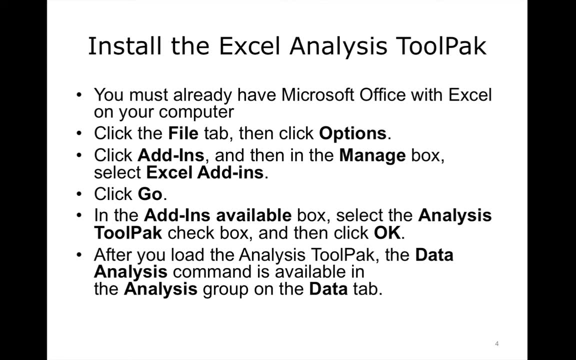 There are also specialized business intelligence applications. Some examples are Tableau, ClickView and IBM's Cognos. For the exercises in this unit, you will use Microsoft Excel because it is widely available. The Analysis Tool Pack is a Microsoft Excel add-in program. 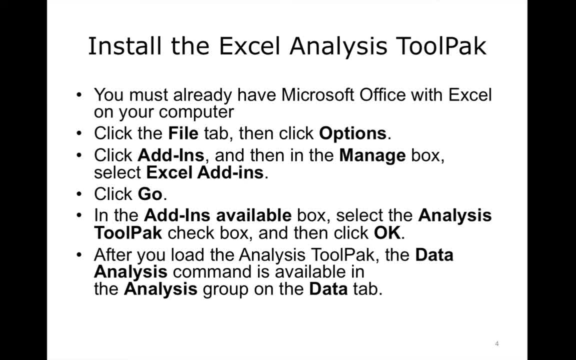 that is available when you install Microsoft Office or Excel. To use it in Excel, however, you need to load it first Open Excel, Click the File tab and then select Options, Click Add-ins and then, in the Manage box, select Excel Add-ins. 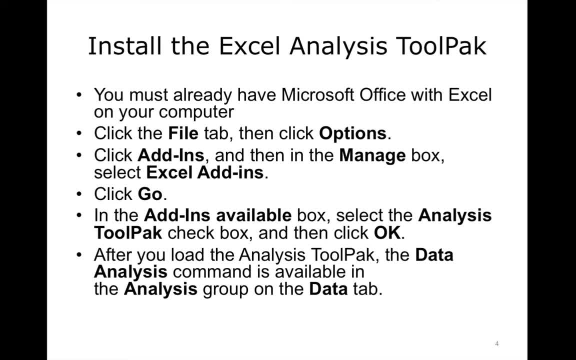 Click, Go In the Add-ins available box, select the Analysis Tool Pack checkbox and then click OK. If Analysis Tool Pack is not available, click Browse to locate it. If you get prompted that the Analysis Tool Pack is not currently installed on your computer, 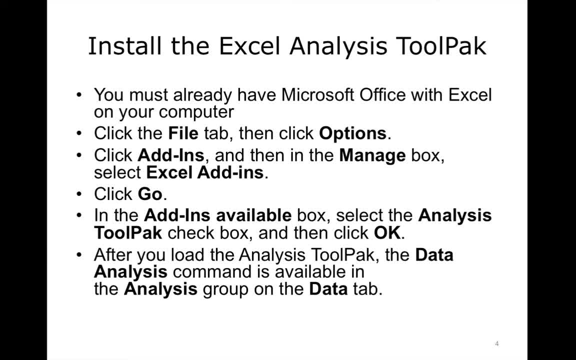 click Yes to install it. After you load the Analysis Tool Pack. the Data Analysis command is available in the Analysis group on the Data tab. Note To include Visual Basic for Application functions for the Analysis Tool Pack. you load the Analysis Tool Pack: hyphen VBA add-in. 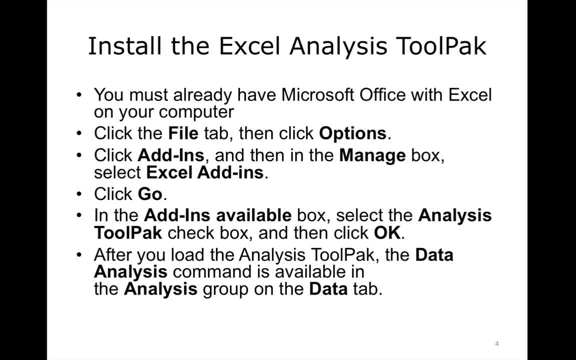 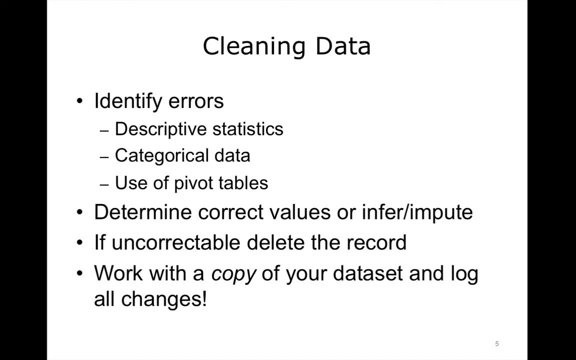 the same way that you load the Analysis Tool Pack. In the Add-ins available box, select the Analysis Tool Pack hyphen VBA checkbox and then click OK. Most, if not all, data sets contain errors or empty fields. These can be due to a wide variety of reasons. 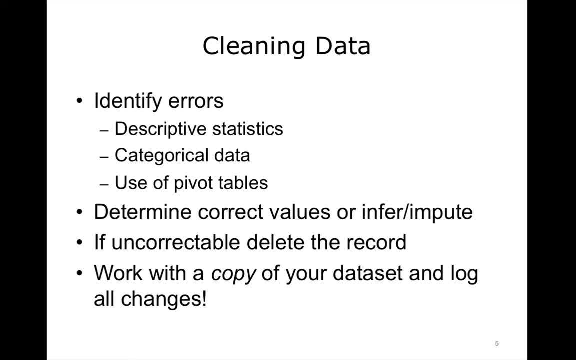 such as keyboard errors or fields left blank because the patient could not provide the information. Before you start doing any analysis, you must examine your data, identify any problems and determine how to address them. The first task is to identify the errors. You can run descriptive statistics. 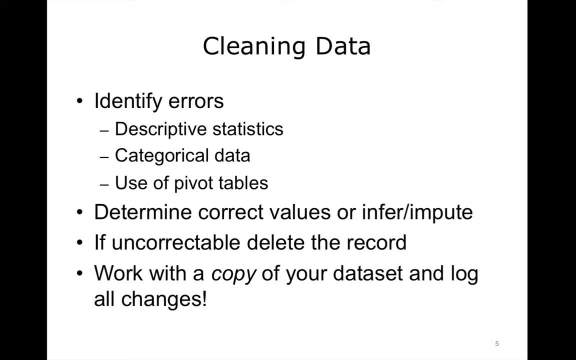 check counts of categorical data and create pivot tables to examine your data. If, or rather when, you find errors or blank entries, you have to decide what to do. Can you determine the correct value from another source, For example, if the patient's height is missing? 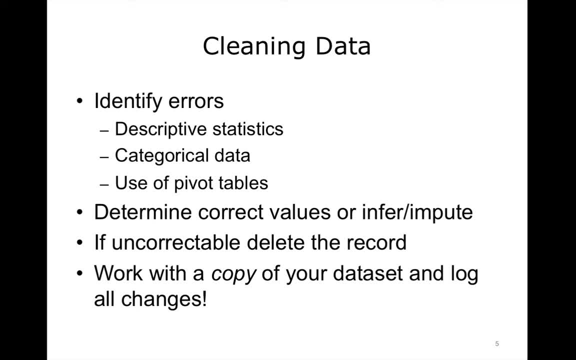 but you have the medical record number. can you look it up on another system? You may also have to infer or impute values. Perhaps the gender field on your patient is blank and you cannot determine the gender from the name. but you see that the patient had a diagnosis of prostate cancer. 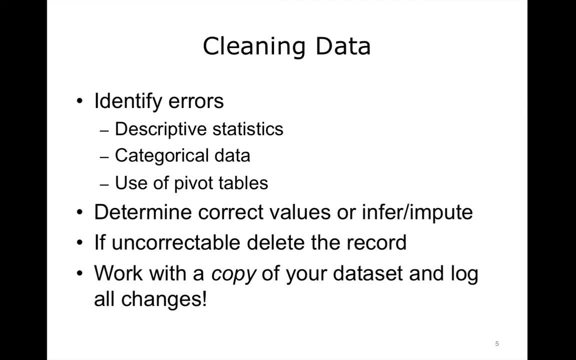 You retrieve a pathology report and see that this is your patient and can therefore safely change the blank gender field to male. If you cannot correct the record, then you may have to make the decision to delete the record from your data set. Good data governance principles are beyond the scope of this unit. 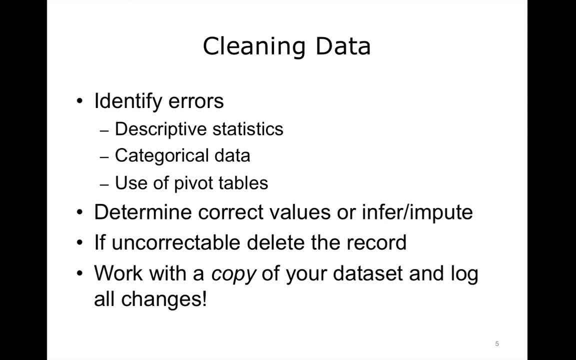 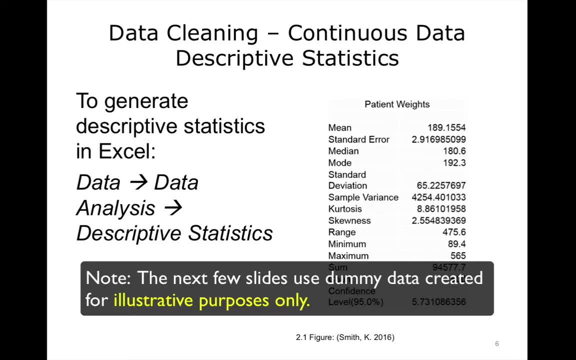 but in general, always work with a copy of your original set of data and keep a record, or log, of every change you make on your data. Now let's take a look at descriptive statistics, which give a basic overview of the data, including the mean or average. 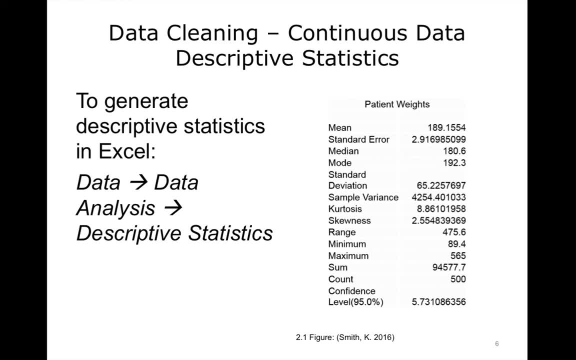 the median or the midpoint, and the mode, the most frequently occurring value, the smallest and largest values and the total number of records. Running descriptive statistics is an excellent way to quickly check if the values are reasonable. For example, this set of data of 500 patient weights. 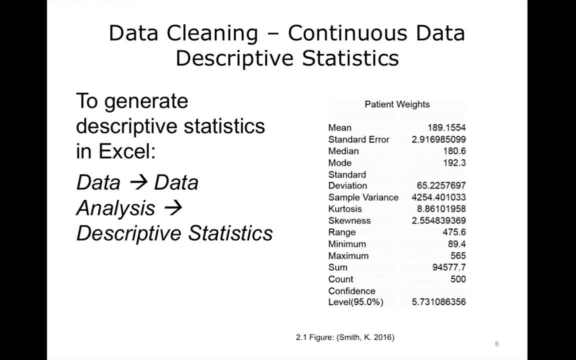 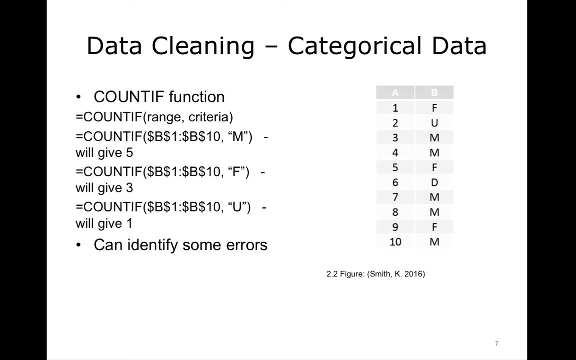 shows a mean weight of 189 pounds, with a minimum of 89 and a maximum of 565.. To generate descriptive statistics in Excel, click Data, then Data Analysis, then Descriptive Statistics. You will probably have data that is not numeric. 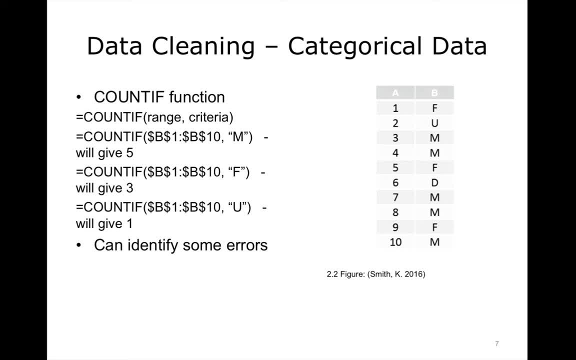 and so counts of how many times certain values occur can be very helpful in not only understanding the data, but also to identify errors in the data. Take a look at this list of 10 patient genders If we use the COUNTIF function on the range of cells. 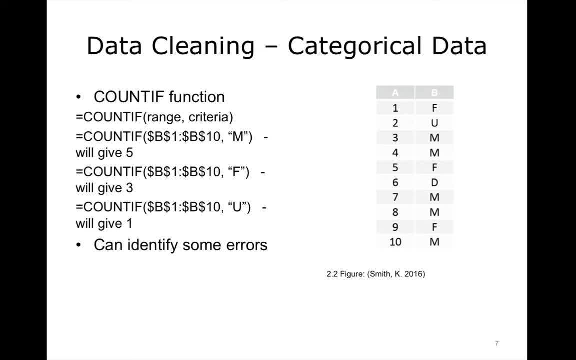 from B1 to B10, and specifically that we want to know how many M's there are. we will get 5.. For entries of F, for female, we will get 3, and for U or unknown, we will get 1.. 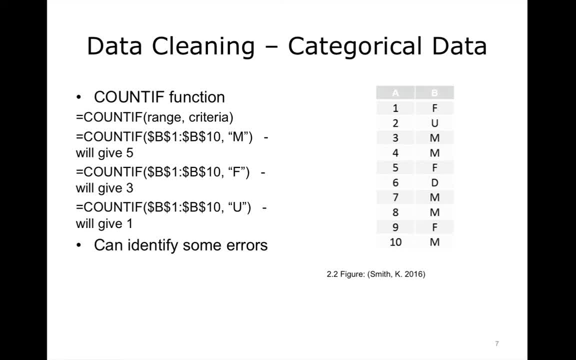 Now we have a problem: 5 plus 3 plus 1 only adds to 9, and we have 10 records. Obviously, in this example we can see that there is an entry with a D in it, which may have been a data entry error. 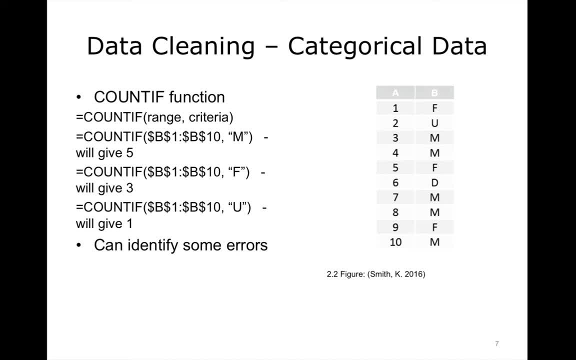 But if we were working with thousands or millions of records, we would not be able to scroll through a list and look for the incorrect records. We need additional tools, So let's look at another Excel tool called Filter. Excel's Filter function lets you display on the screen. 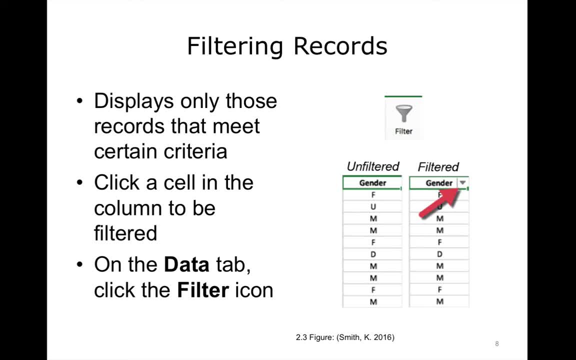 records that meet certain criteria. To filter records, click a cell in the column to be filtered- In this case, we are using the Gender column- And then click the Filter icon on the Data tab. Nothing will appear to happen, other than a drop-down arrow will now appear. 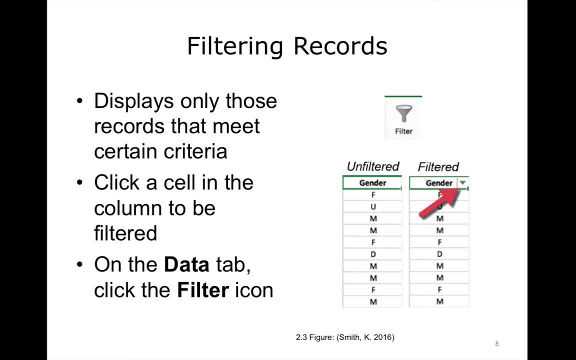 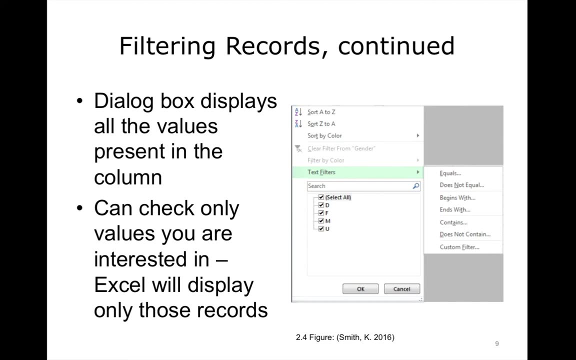 at the right-hand of the column heading, indicated here with a red arrow. Click the drop-down arrow and we'll look at what happens on the next slide. If you click the drop-down arrow on the column header, you should now see a dialog box with several options. 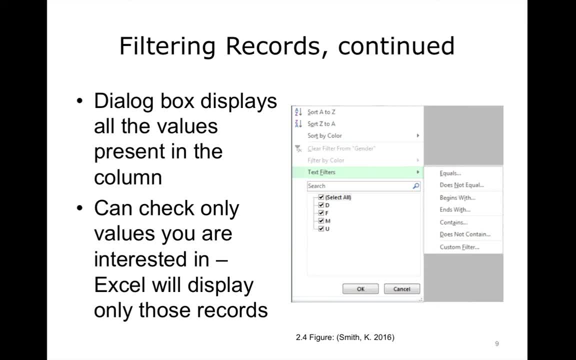 First, at the bottom of the dialog box, is the list of all the values that were present in the Gender column: the M, F, U and the D. that is an incorrect value. To see only the records with a- D in the Gender column. 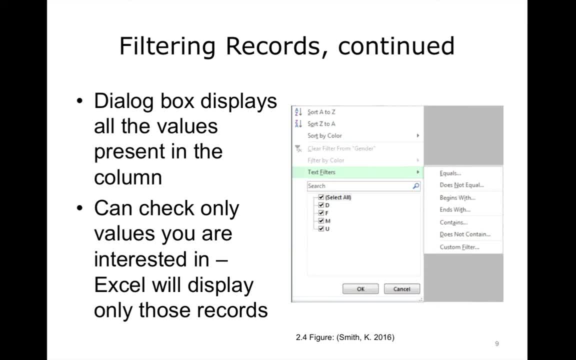 uncheck the F, M and U and leave only the D checked. You can also specify additional filtering criteria, such as whether the entry in a cell equals a value, does not equal a value, begins or ends with a string of characters, and so on. 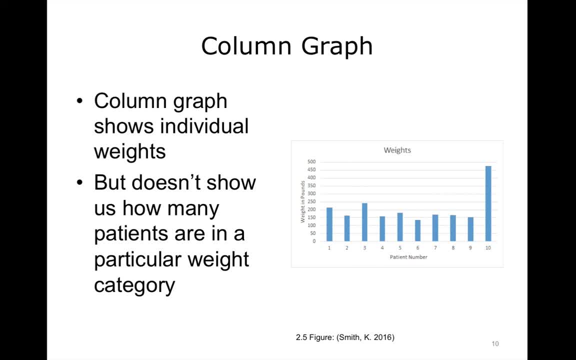 Let's take a look at the weights for these 10 patients. We could graph them, but this isn't particularly helpful. Individual weights on a graph, plotted against patient number, doesn't give us insight into the number of patients that we're going to be looking at. 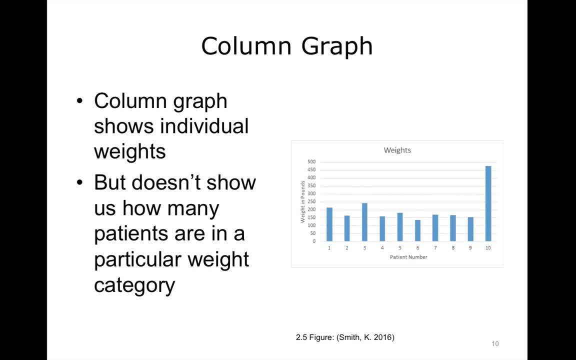 We could graph them, but this isn't particularly helpful. Individual weights on a graph plotted against patient number doesn't give us any insight into categories of weights such as one category for 200 to 249 pounds, another category for 250 to 299 pounds and so on. 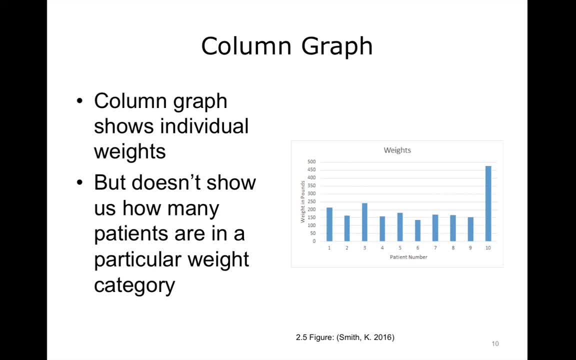 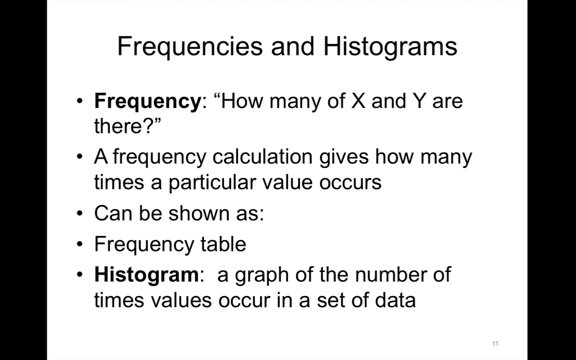 That's a job for a frequency histogram which looks like a column graph but shows distributions. Let's look at frequencies in histograms now. Frequencies answer the question: how many of something is there? Recall that. nominal data are things like names, labels or categories of data. 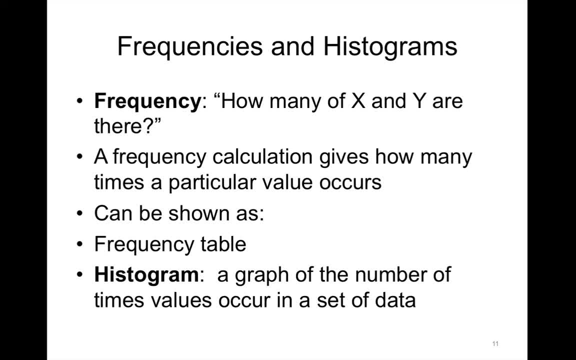 Examples of nominal data are patient names, genders- such as male, female and unknown- and marital status: married, single, divorced, widowed. Frequencies are primarily shown in a table format and also in a histogram which looks like a column chart, so don't get confused. 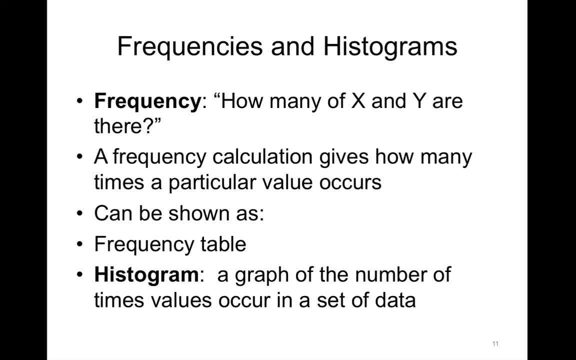 A histogram is a graph of the number of times values occur in a set of data, in other words, the frequency of the values. It looks like a column chart in that it is a visualization of the distribution of values. Let's look at an example now. 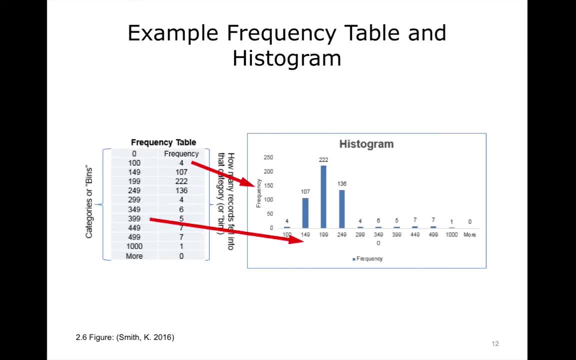 On the left is a frequency table and on the right is a histogram of the same data. The categories or bins from the frequency table are the numbers along the horizontal- x-axis of the graph, and the frequencies or counts are the numbers along the vertical or y-axis of the graph. 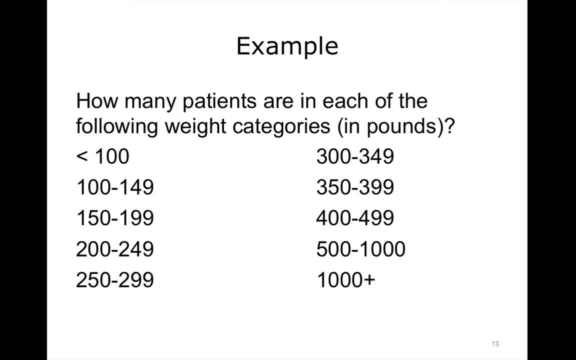 Let's step through the process of creating that table and histogram. We want to know how many patients fall into each category and then we want to see this as a graph. We'll take our 500 patient weights and set up categories in roughly 50-pound divisions. 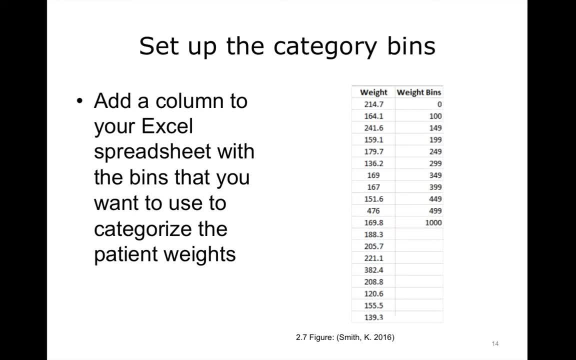 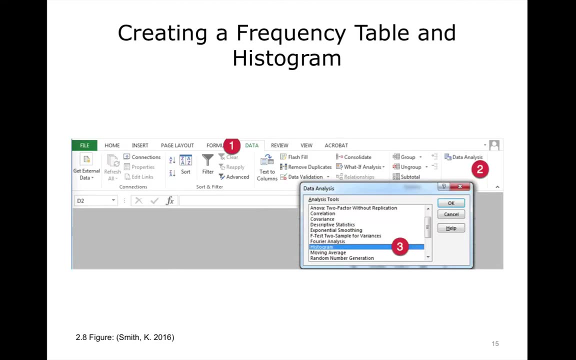 Add a column to your Excel spreadsheet with the bins that you want to use to categorize the patient weights. Note that in this example only a few of the 500 patient weights are shown. To run frequencies in Microsoft Excel, click the Data tab, then click Data Analysis. 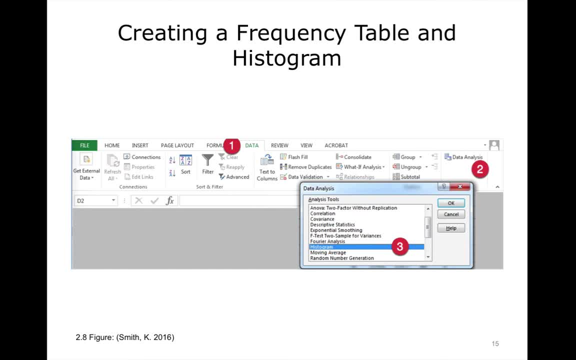 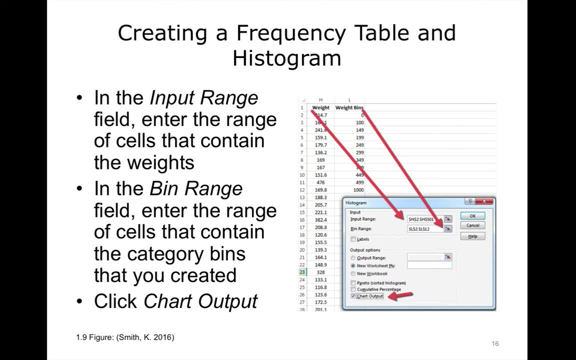 and then choose Histogram. In the Input tab, enter the range of cells that contain the weights, in this case the data in H2, and continue through H501.. In the Bins Range field, enter the cells that contain the category bins that you created. 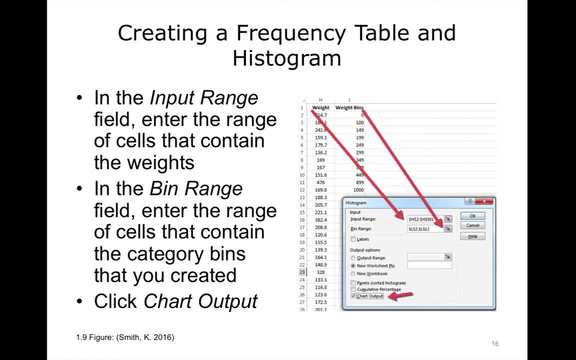 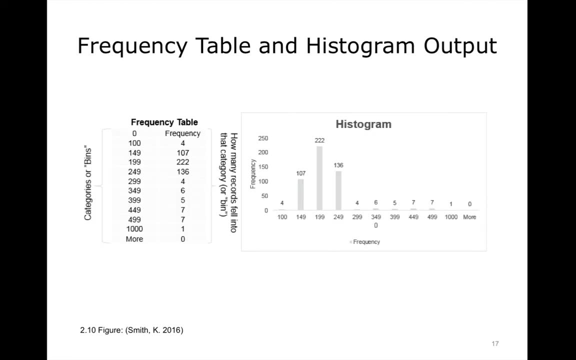 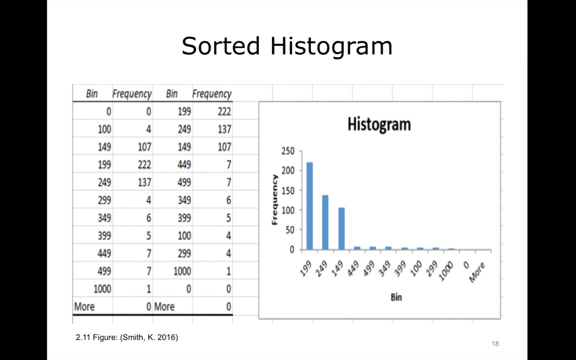 In this example, the bins are in cells L2 through L12.. Finally, determine what type of output you want. Let's click Chart Output for this example. Excel will produce a new worksheet in your file with a table on the histogram Sorting. the histogram organizes the categories or bins. 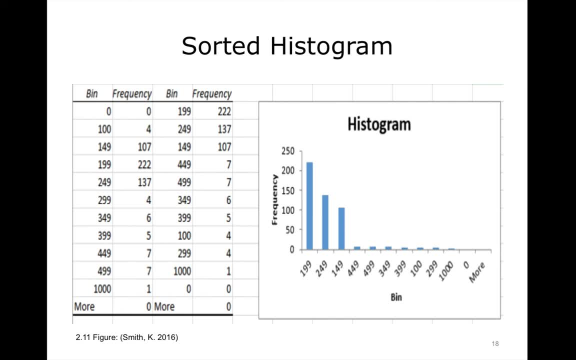 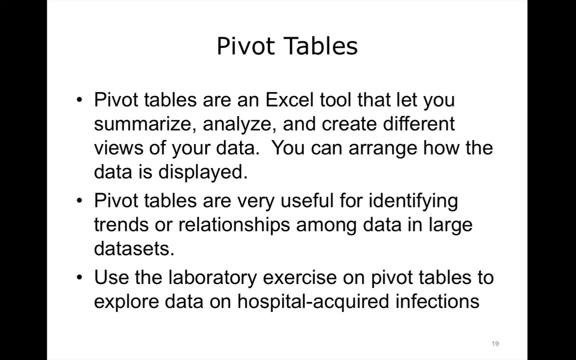 by how often they occur. The most frequent bins will be to the left of the graph. Pivot tables are an Excel tool that you. Pivot tables are an Excel tool that let you summarize, analyze and create different views of your data. You can arrange how the data is displayed. 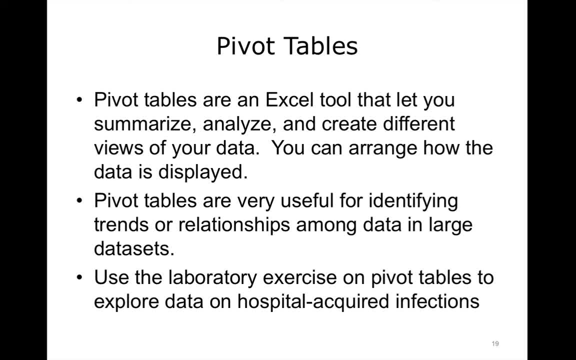 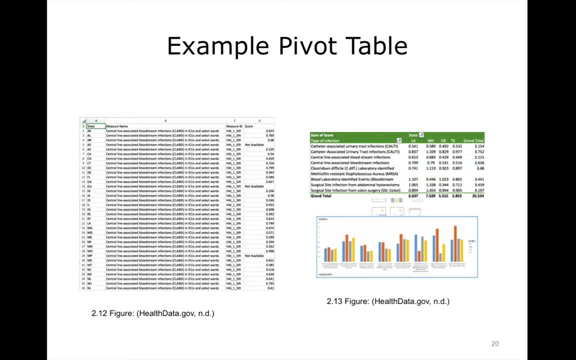 Pivot tables are very useful for identifying trends or relationships among data in large data sets. Here is an example of a raw set of data on the left and a pivot table of some of the data on the right, along with a column chart of the data in the pivot table. 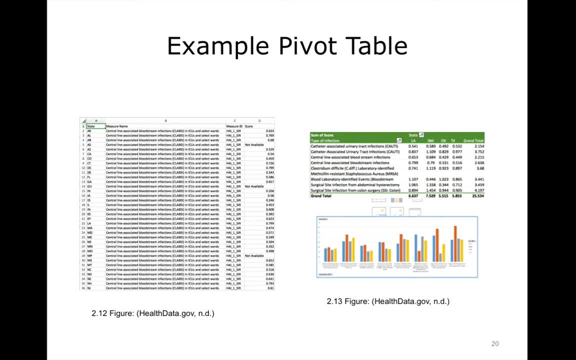 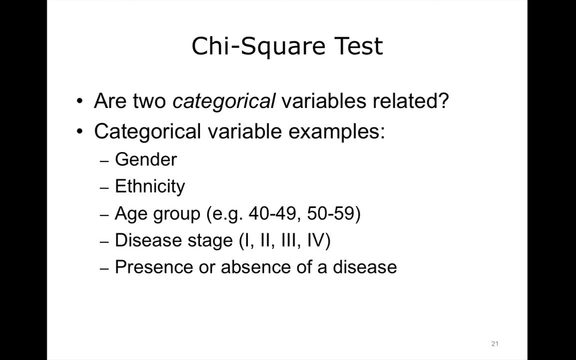 You can practice creating this table in the laboratory activity associated with this unit. Now think back to the section in this component on types of data. Recall that we discussed nominal, ordinal, interval and ratio data. Nominal data included things that were names or categories. 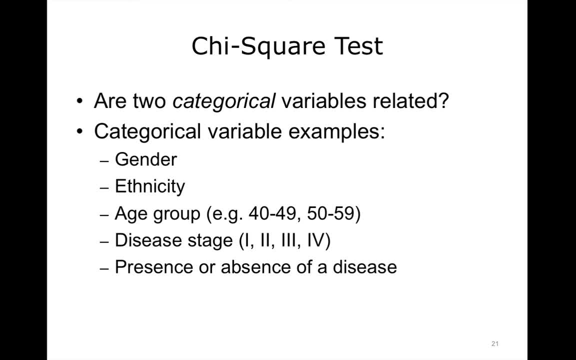 such as gender, race, religion, smokes yes or no, and so on. Another name for nominal data is categorical data, and this term is typically used in statistics. So think about the example of gender. Let's say that we have three categories. 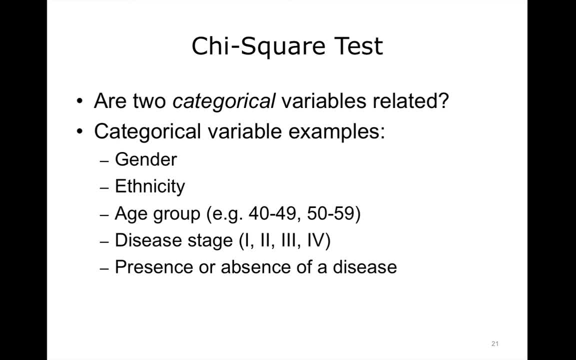 male, female or unknown. You can do simple analysis, such as counting how many of each type of gender in the hospital, but it doesn't make sense to do many kinds of calculations on categorical data, For example. it doesn't make sense to try to calculate. 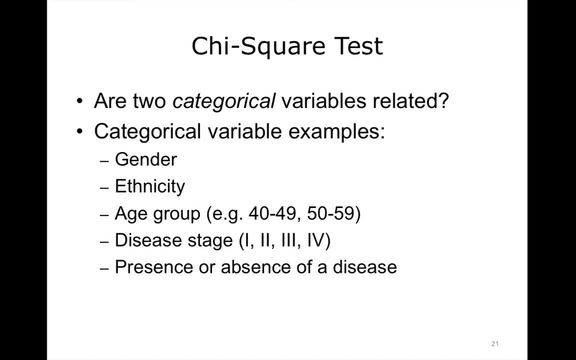 the average gender of the patients in the hospital. However, you may want to know if there is a relationship between two categorical variables. For example, you may want to know if there is a relationship between patient gender. we'll simplify it to just male and female for this example. 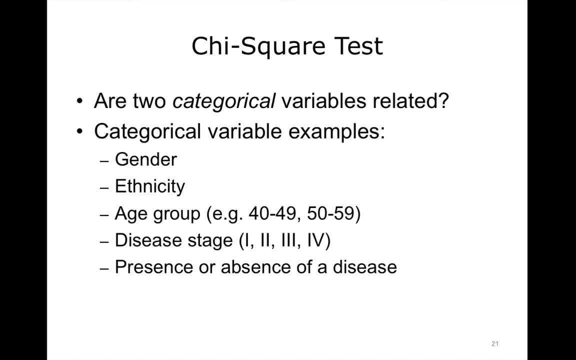 and smoking status. yes, no. The chi-square test is used to determine whether there is a relationship between two categorical or nominal variables. In other words, it checks to see if the two variables are independent of each other. You'll see this frequently reported in literature.